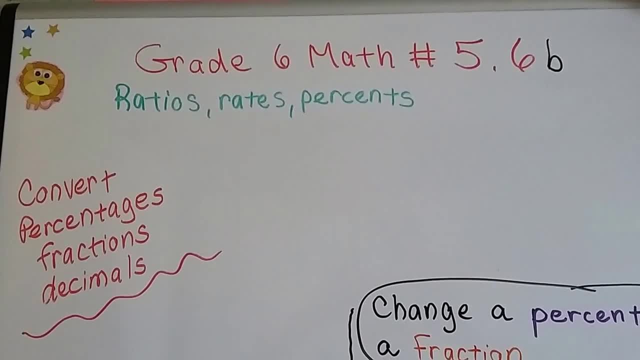 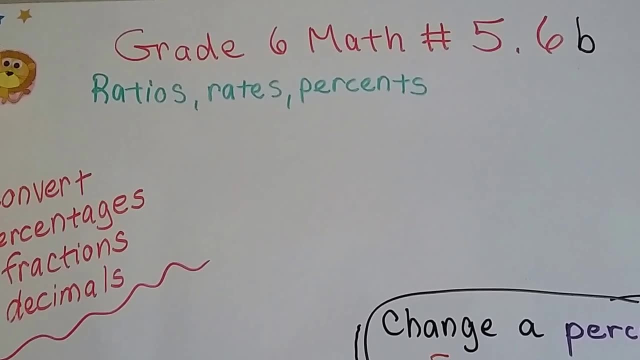 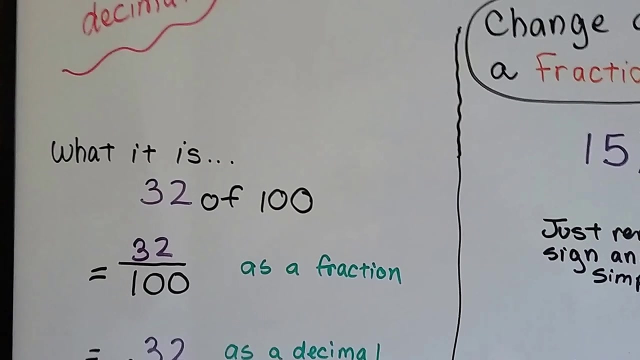 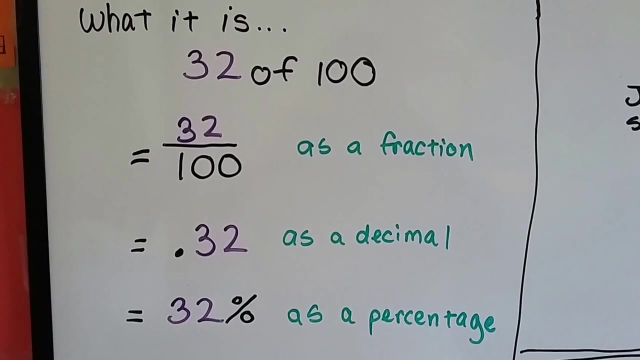 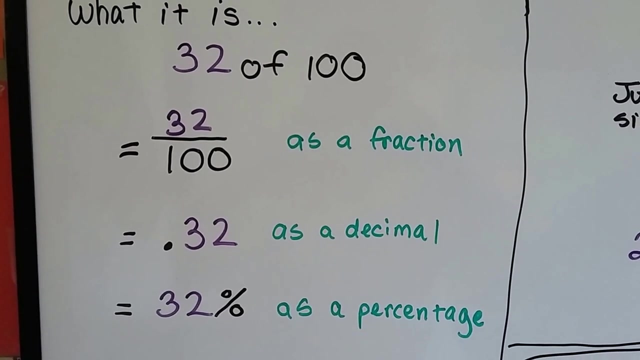 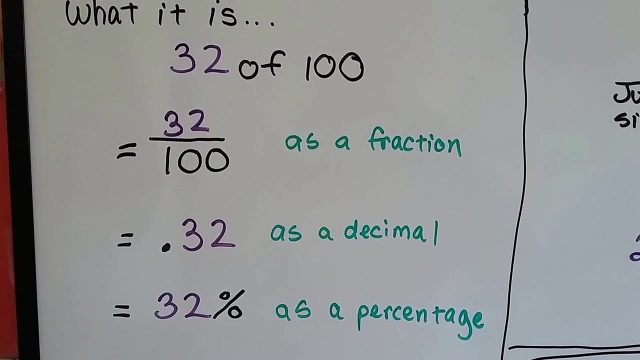 Grade 6 Math number 5.6b: Convert Percentages, Fractions and Decimals. This is a continuation of the previous video 5.6a. You might want to watch that one first. We're going to convert percentages, fractions and decimals back and forth to each other. So to understand, let's look at this first What it is: 32 out of 100 means 32 hundredths as a fraction, .32,, 32 hundredths as a decimal or 32% as a percentage. See 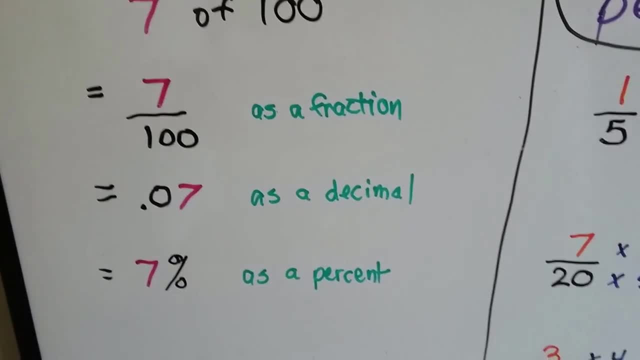 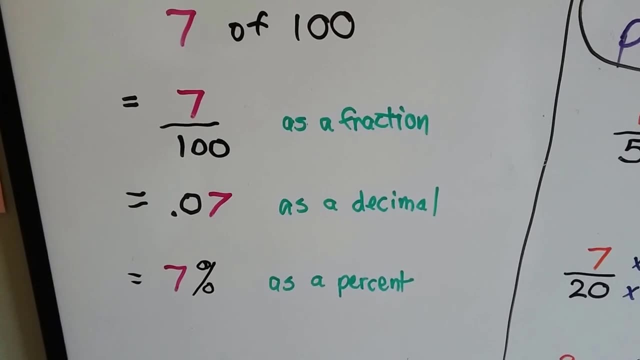 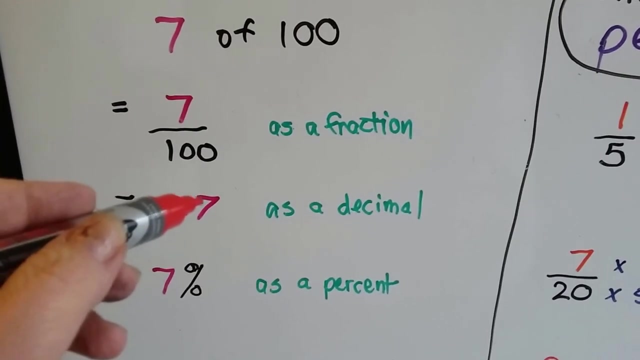 Let's try another one that's smaller. 7 out of 100 would be 7 hundredths as a fraction, .07 as a decimal. We now had to put a 0 in the tenths place to hold it as a placeholder, because this is hundredths. 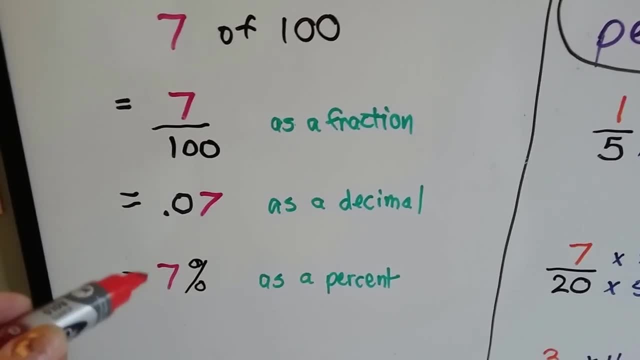 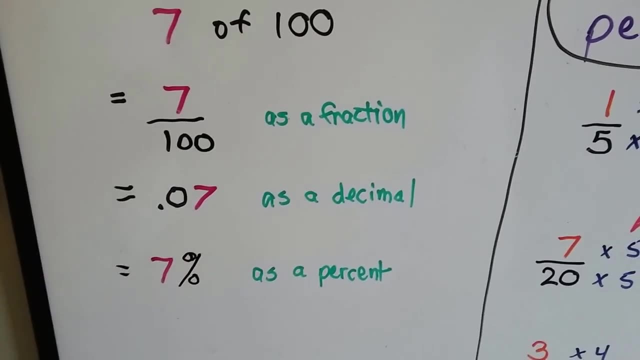 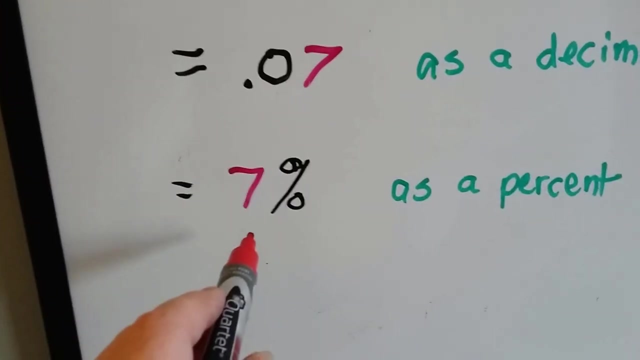 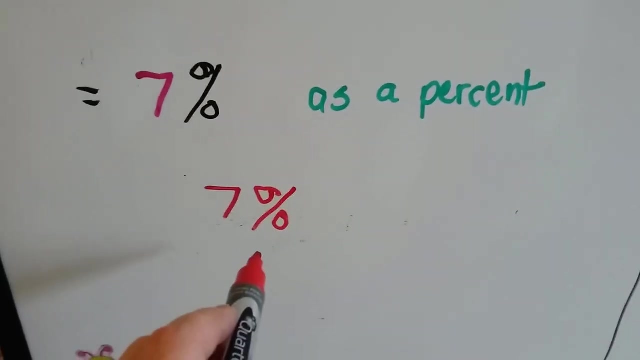 And it's 7%, It doesn't need the 0. if it's a percentage, It doesn't need the 0 in front like a decimal does. This percentage sign pretty much means it's part of 100. Sometimes you can look at it as the 7% is almost like, because there's a 0, a line and a 0. It's like someone got crazy and forgot how to write 100, and there's a 1 and a 0, 0.. 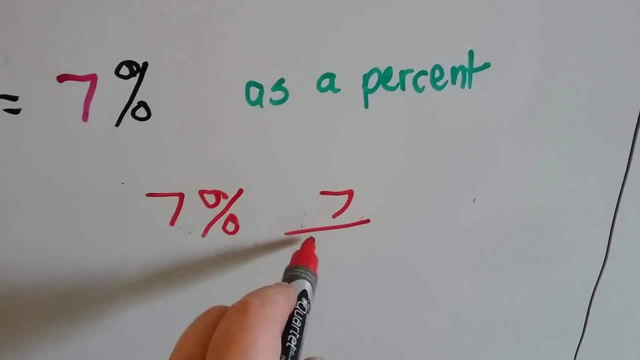 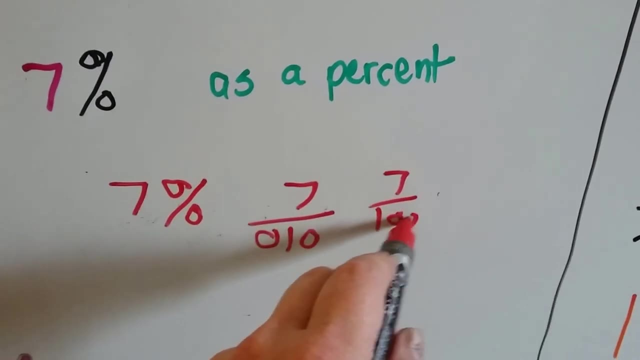 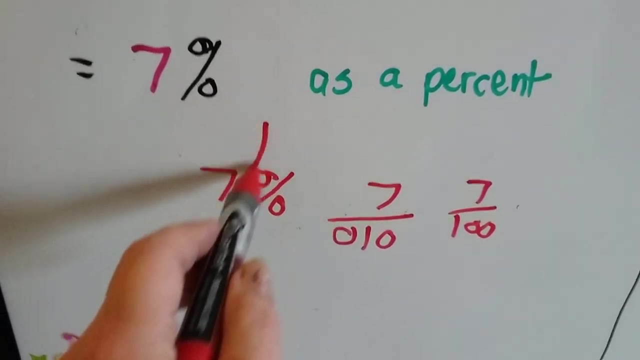 So the 7% is like 7 over this crazy you know mixed up 100, and it's supposed to be 7 over 100. So you can kind of look at it as 7 over 100. And that the 100 is written all crazy. See, It's 7 over 100. See. 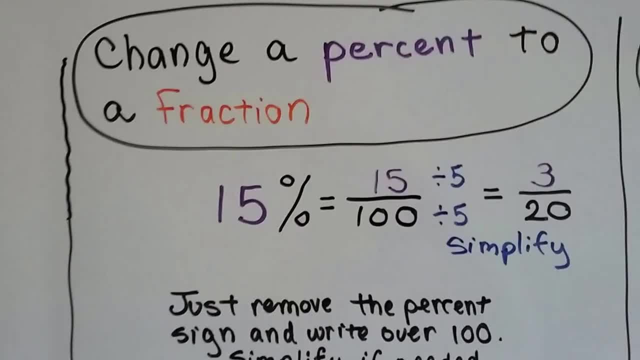 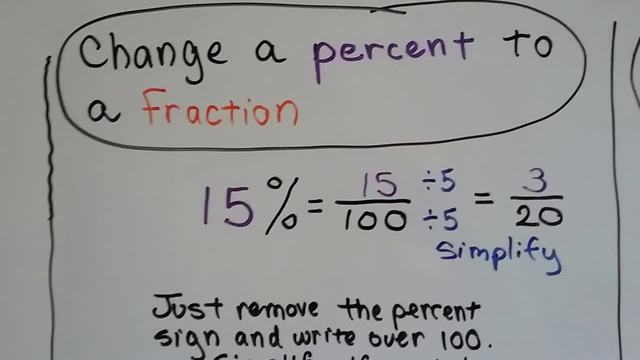 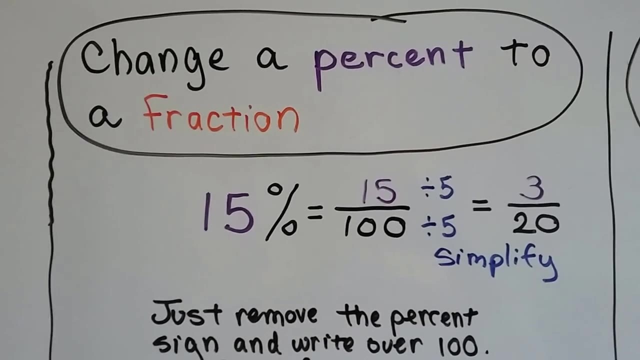 Alright, To change a percent to a fraction. if we've got 15% and we want to change it to a fraction, 15% means 15 parts of 100. So we just write the 15 over the 100. But we need to simplify them. You can't just leave them. We're not done. 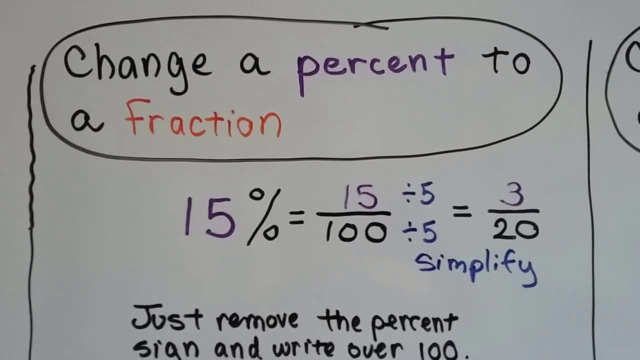 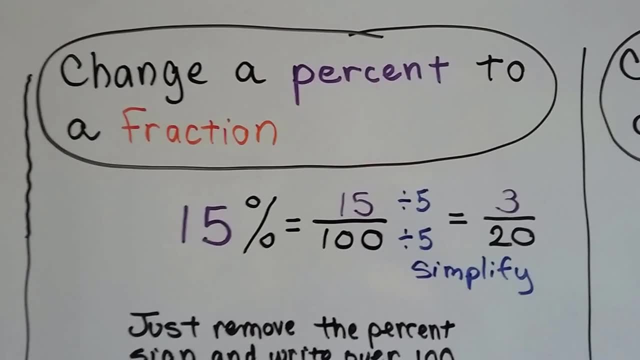 What can go into 15?? You can write 15 and 100 equally, So I tried 5.. 15 divided by 5 is 3, and 100 divided by 5 is 20.. So I got 3 20ths and that's as low as it can go. 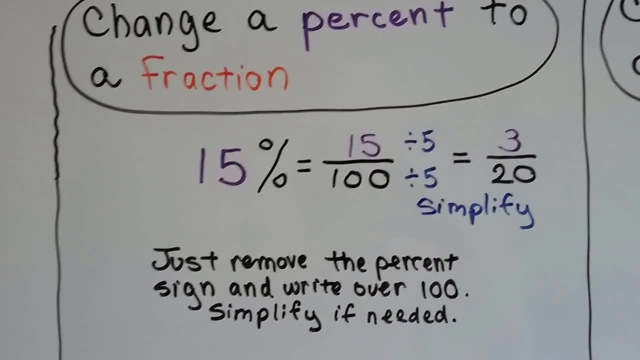 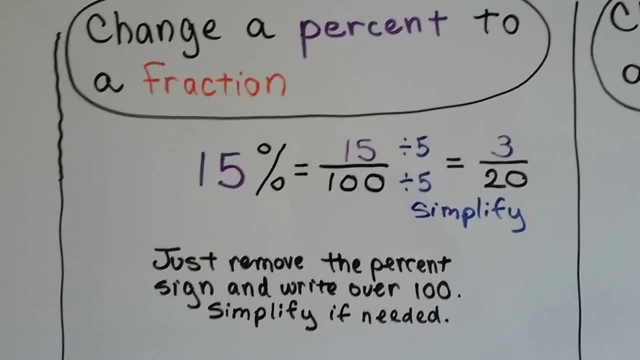 So just remove the percent sign and write over 100.. See, I wrote the 15 over the 100. And then simplify if needed. Okay, That's an easy one. Here's 25%. It's written as 25 over 100. 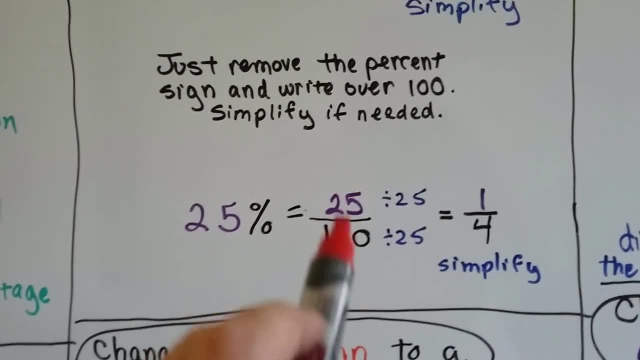 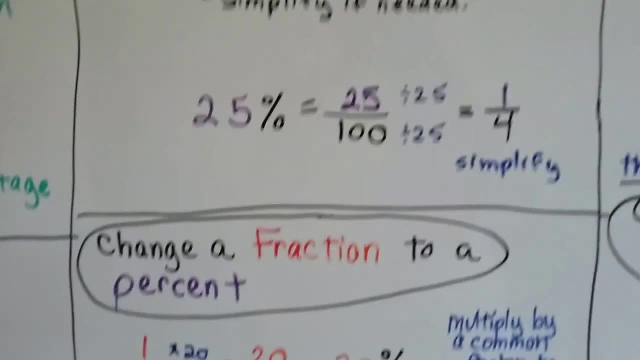 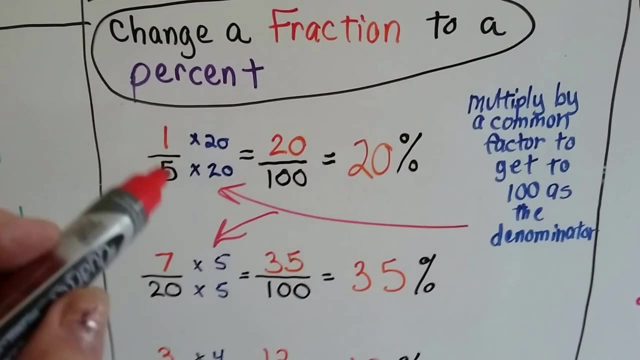 I divided the numerator and denominator by 25, because they know they both go into each other, and I got 1, 4th. See It's like 25 quarters and a dollar. See Now to change a fraction to a percent. if you have 1, 5th before we can do anything and change it to a percent. 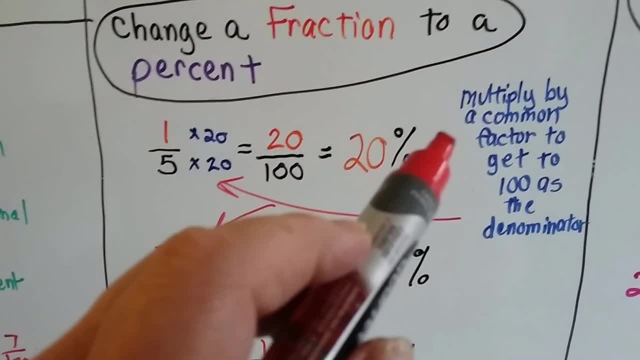 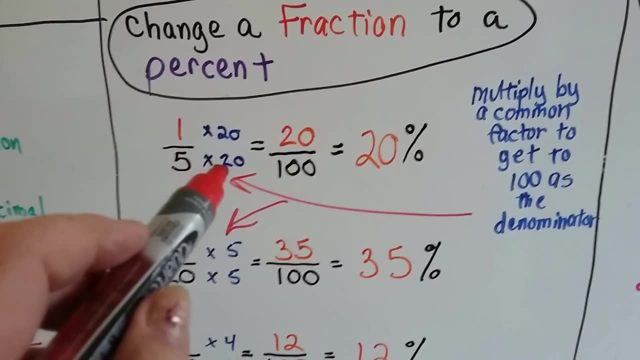 we need to make the denominator 100. We need to multiply by a common factor to get 100 as the denominator before we do anything. So the 5 can be multiplied by 20. So we have 20 to become 100. The numerator gets jealous. He gets multiplied by 20.. 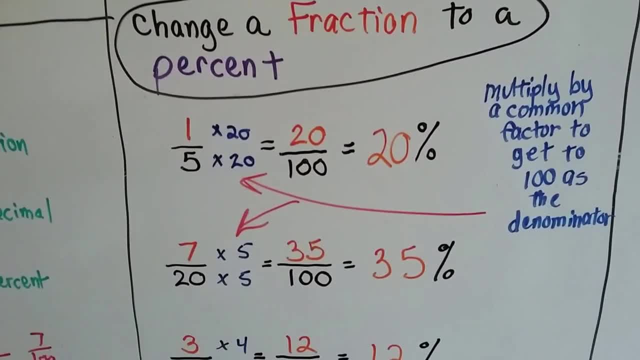 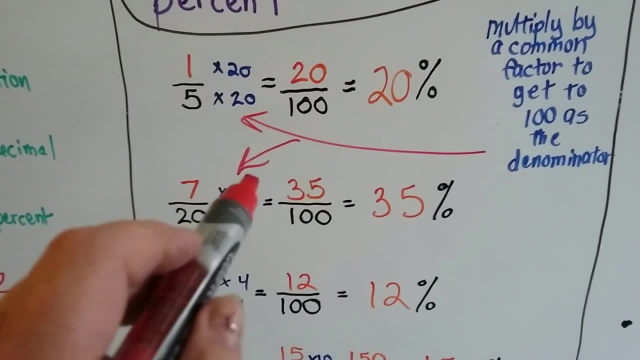 Now we've got 20 over 100. And we just write that as 20%. If we have 7 20ths, see, We know it could be multiplied by 5.. So the 7 gets multiplied by 5. And we have 35 over 100. 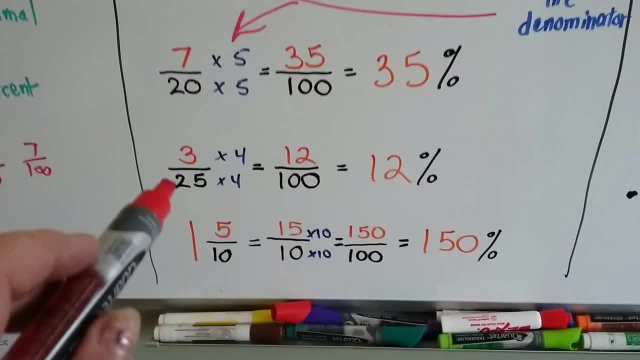 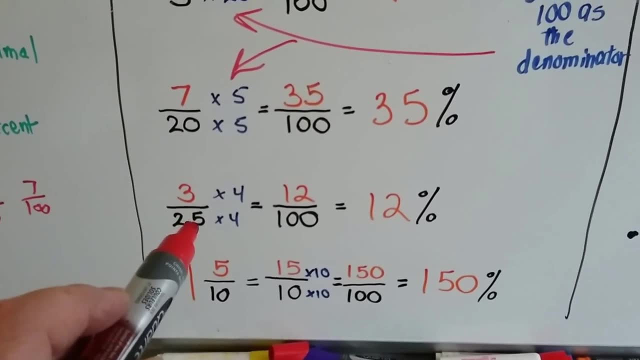 And we just write it as 35%, See, Because we know this is 35 hundredths 35 parts of 100.. If we have 3 25ths, we know 4 25ths makes 100.. See, Because we know this is 35 hundredths 35 parts of 100.. If we have 3 25ths, we know 4 25ths makes 100. 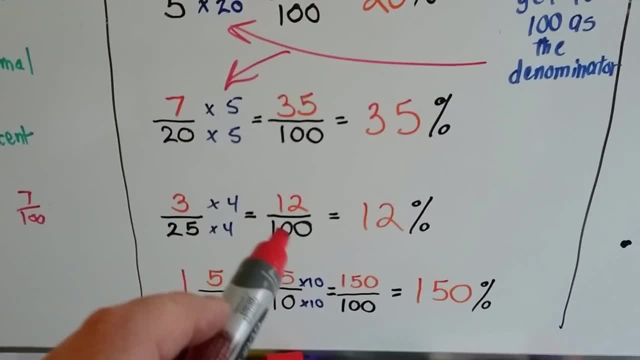 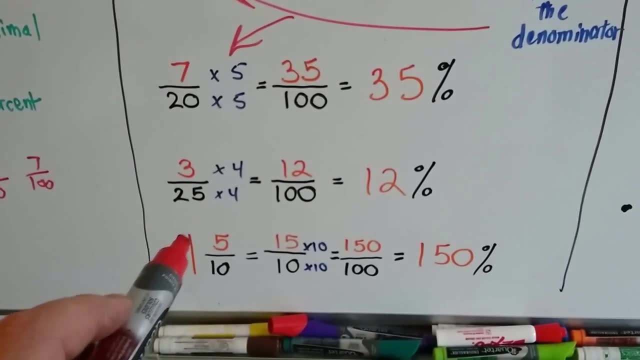 So the 3 has to be multiplied by 4. It becomes 12 over 100.. Now we can write it as a percentage, Because we've got it as hundredths: It's 12%. What if we've got 1 and 5 tenths? 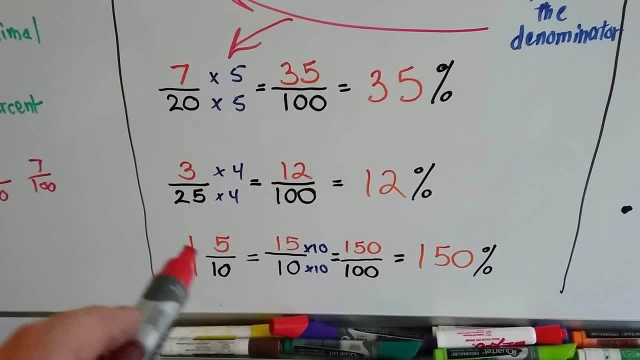 Well, we need to convert it to an improper fraction. Well, we need to convert it to an improper fraction: 1 times 10 is 10 plus 5 is 15.. 1 times 10 is 10 plus 5 is 15.. 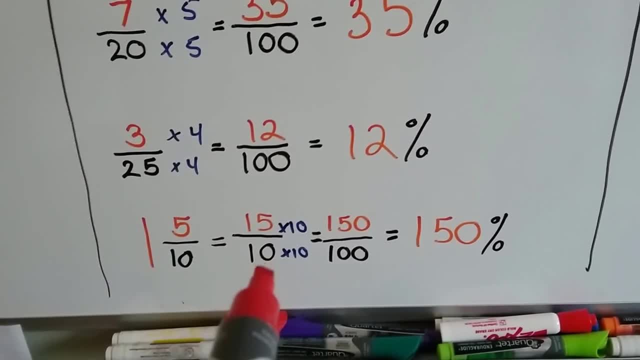 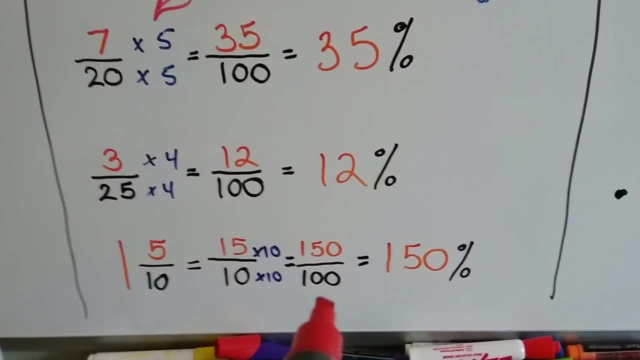 Now it's 15 over 10.. We need to get this 10 to 100. So we multiply them both by 10.. Because 10 times 10 is 100. So 15 gets multiplied by 10.. So now it's 150 over 100.. 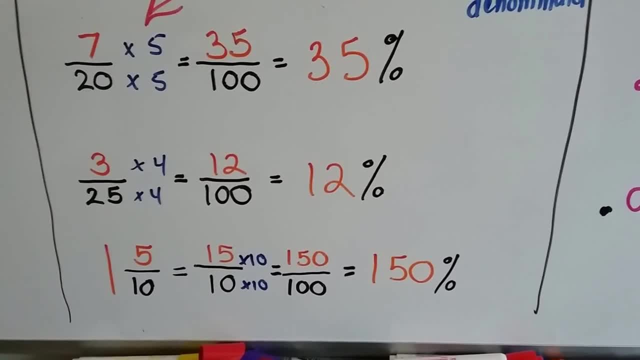 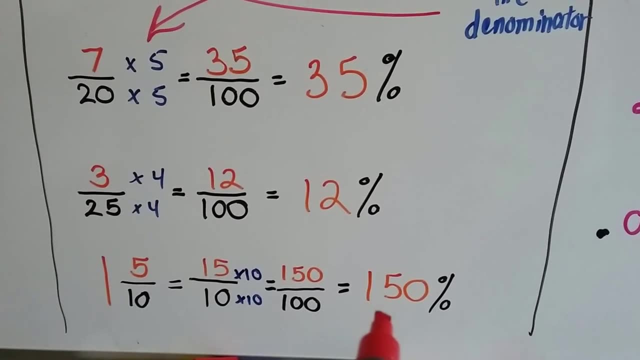 And it's 150 percent, See. So, whatever it is over 100, that's what the percentage is, And we know that 150 percent means 1.5, or 1 and 5 tenths, Or 1 and 50 hundredths. 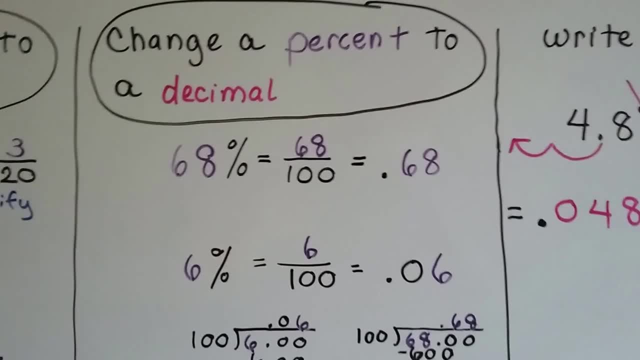 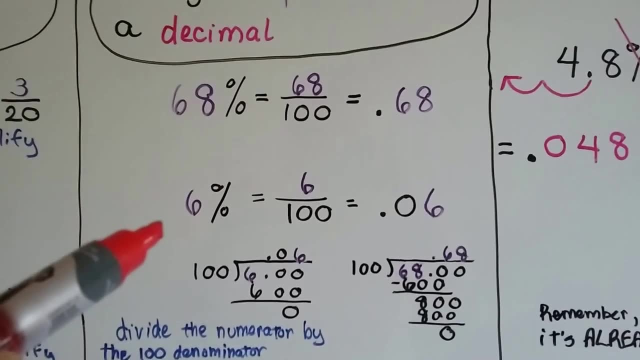 It's all the same To change a percent to a decimal If we've got 68 percent and we want to change it to a decimal. this one is actually kind of weird. What we do is we divide the numerator by the denominator. 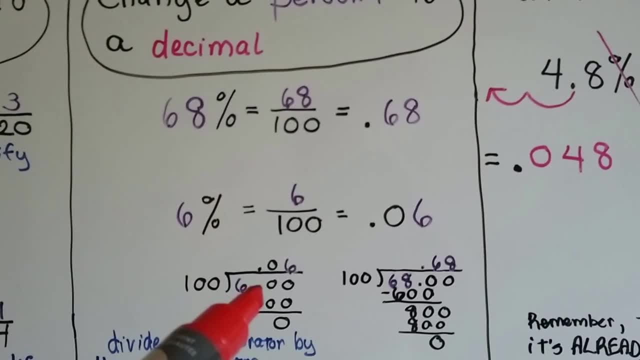 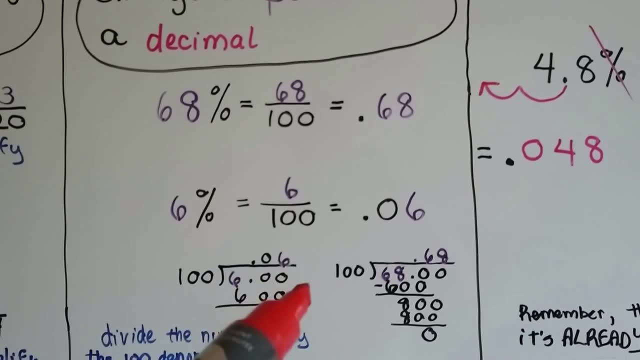 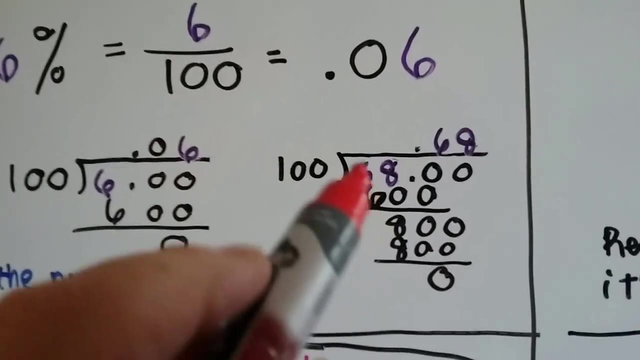 We actually put the little tiny numerator on the inside as the dividend, And the 100 becomes the divisor, And if it doesn't fit, we have to add a decimal point in zeros. So, in order to do 68 over 100, what I did was: 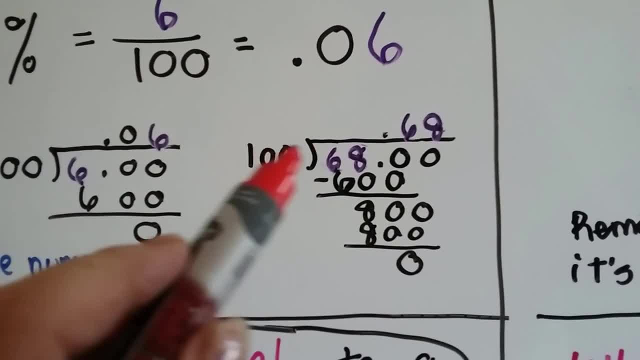 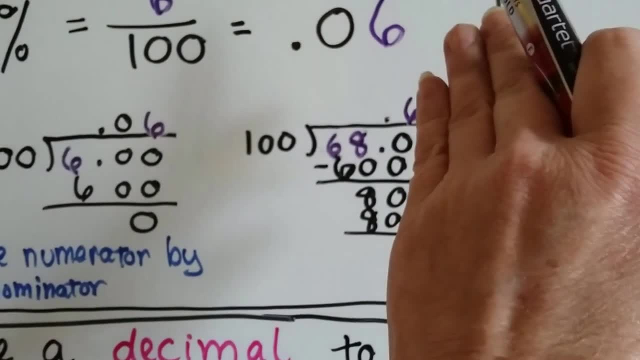 I put the 68 on the inside. The 100 is the divisor And 100 can't fit into 68. So I put a decimal point in 100. And a zero. Well, 100 can go into 680 six times. 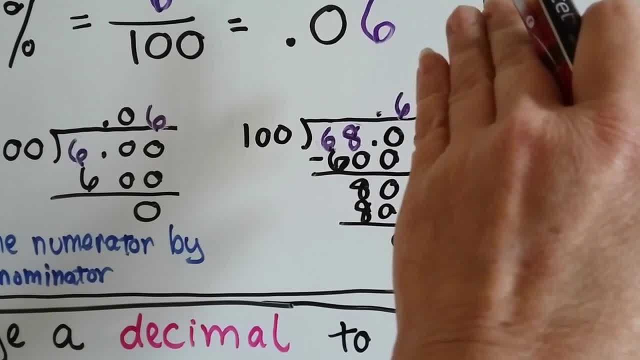 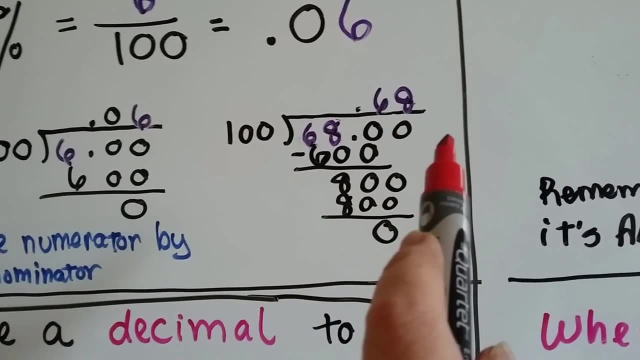 So I did that. 100 times 6 is 600.. I did my subtraction and got 80.. And I had to add another zero, Because we can add as many zeros as we want. after the decimal point. See, It became 800.. 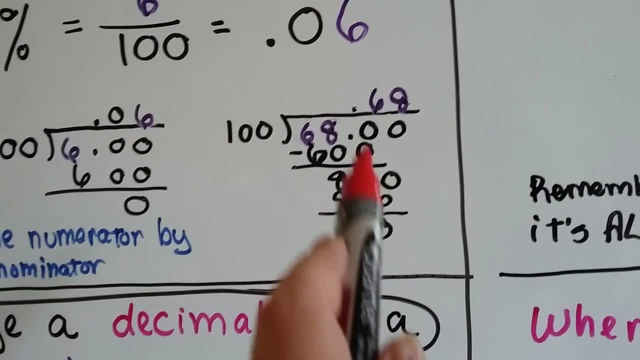 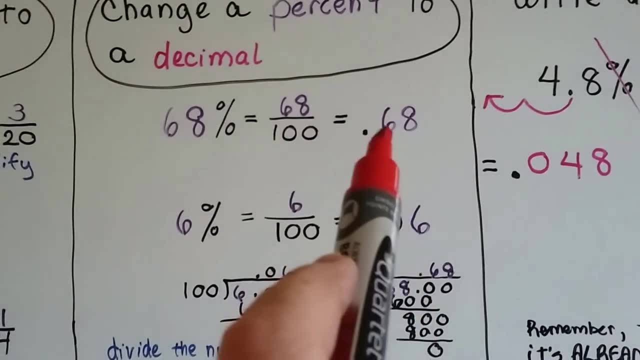 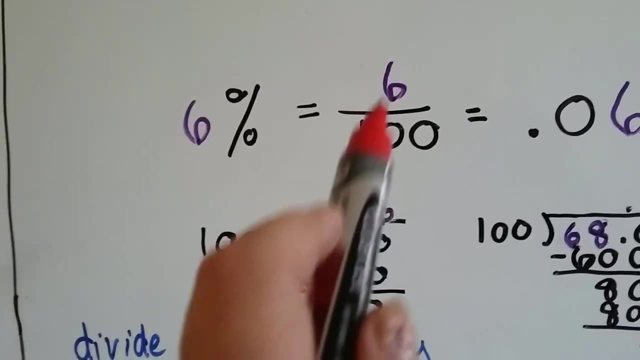 I multiplied 100 times 8.. Subtract It got zero, So that percentage is now a decimal: It's .68.. I did the same thing for 6%. I know it's 6 parts of 100.. So I really could have just written. 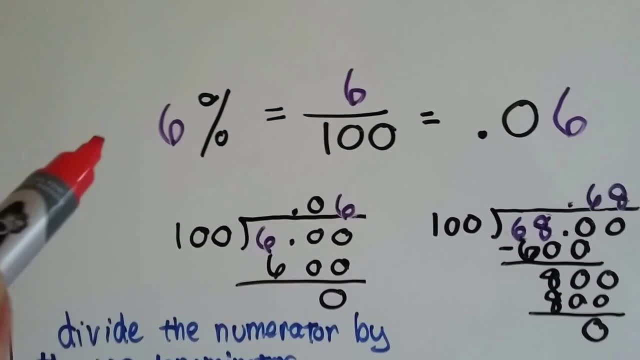 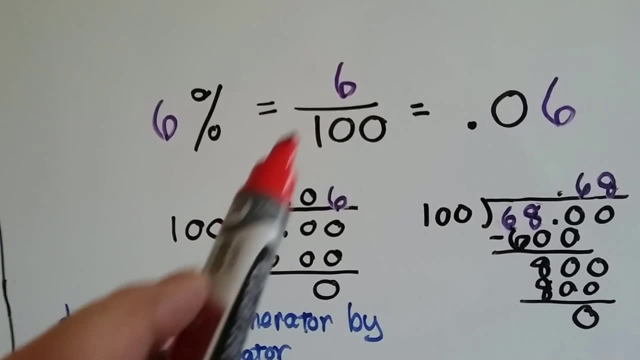 6 over 100, because 6% is 6 parts of 100. But to do it with math, what I did was I made this the dividend and this the divisor, And even though that's tiny and 100 won't fit into it, 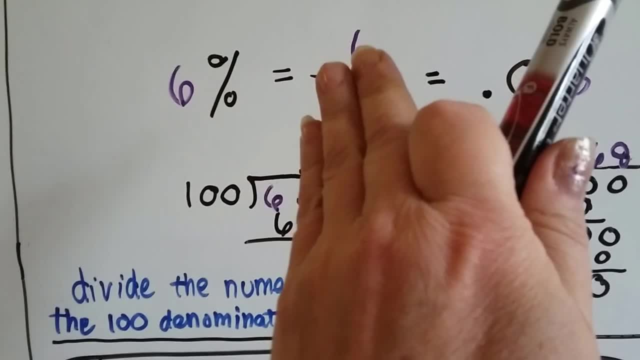 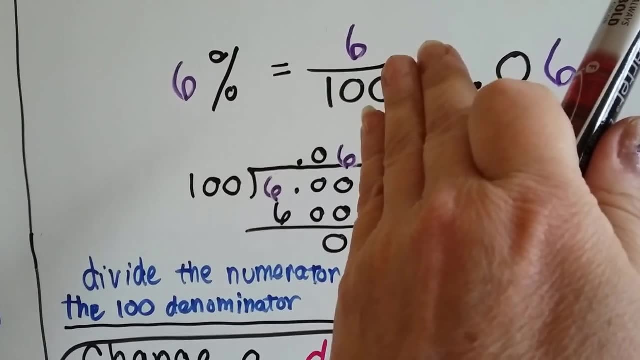 I just added a decimal point and a couple of zeros. 100 can't go into 6.. I added the decimal point and a zero. It can't go into 60, so I added another zero And 100 times 6 is 600. 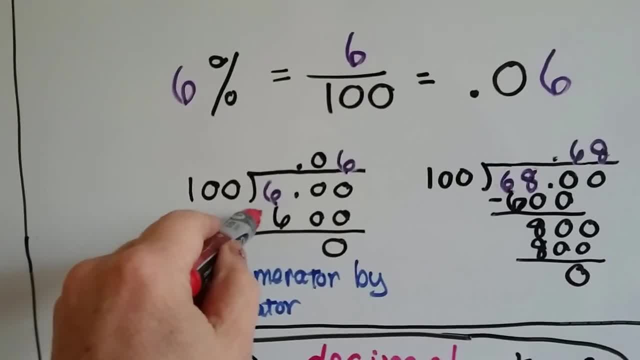 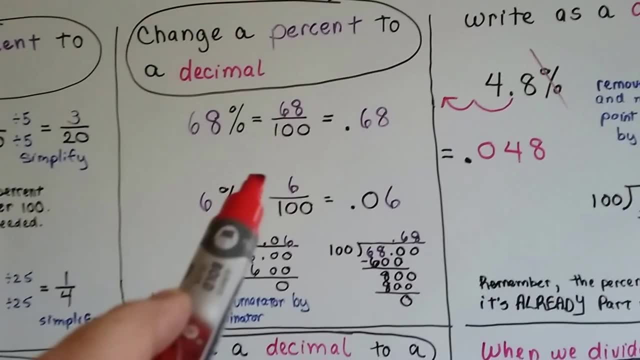 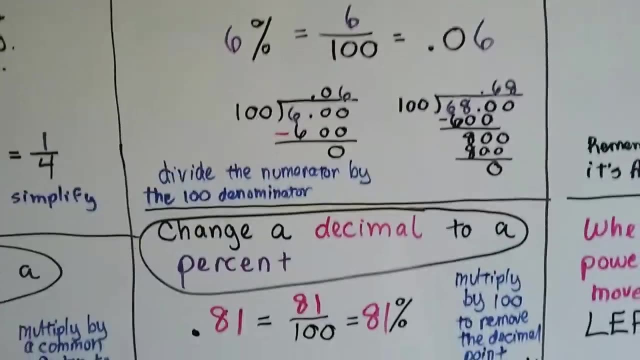 And I subtracted, I got a zero and I knew my answer was .06.. So see, when you're changing a percent to a decimal, you actually divide the numerator by the 100 on the outside, as the divisor See To change. 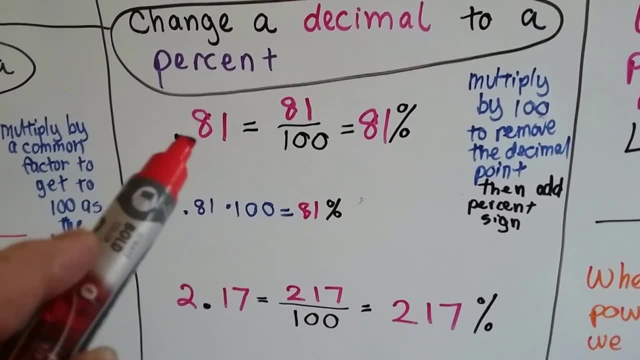 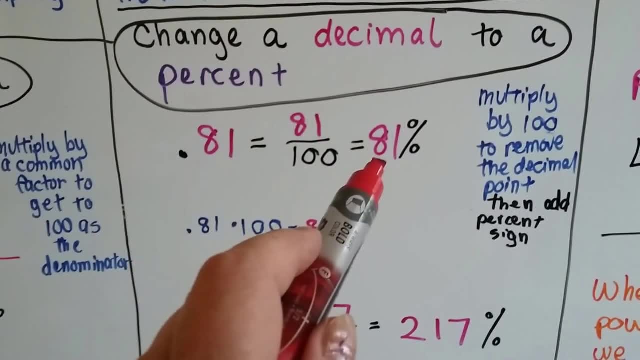 a decimal to a percent. here we have 81 hundredths. Well, we know it's 81 hundredths as a fraction. It's written like that, Which we also know would be 81%. Well, what we're doing is we multiply by 100. 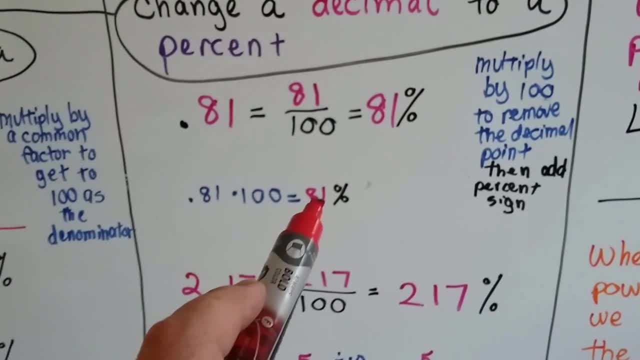 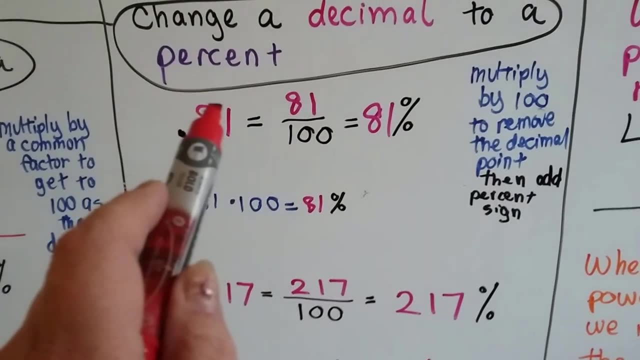 to remove the decimal point. .81 times 100 becomes 81. And then we just add the percentage sign See. So mathematically that's what we're doing In our heads- we can just say: well, it's 81 over 100.. 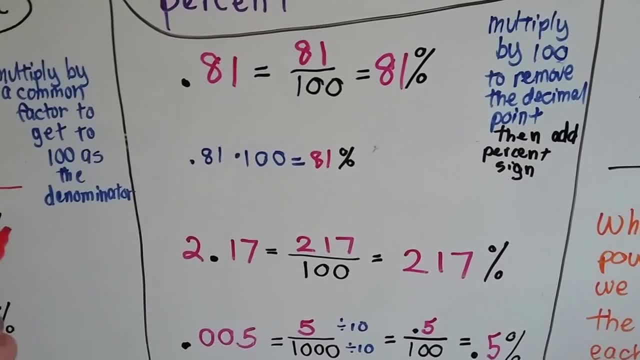 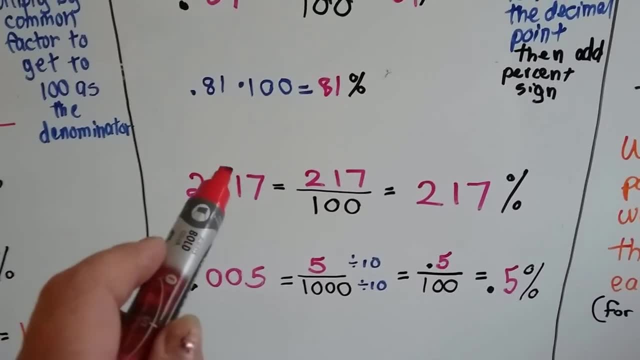 But if someone says, yeah, but mathematically what are you actually doing? You say, oh, I'm multiplying by 100 to get rid of the decimal point. That's the answer If we have 2.17 and we want to change. 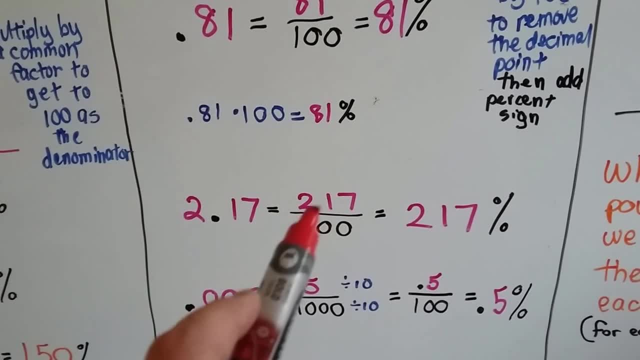 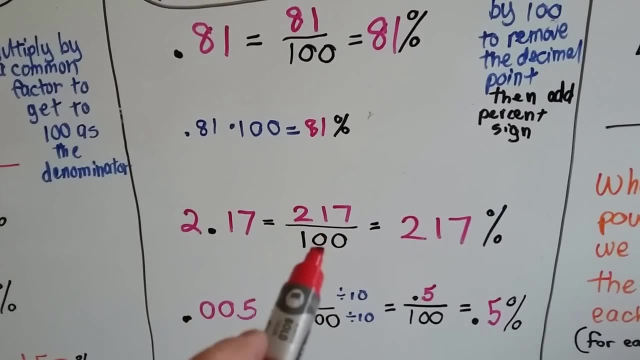 it into a percentage. we put it over 100.. 217 over 100.. See, Because we have 2 whole and 17 hundredths. So it becomes an improper fraction And we know that if we multiply it by 100 that we would get 217%. 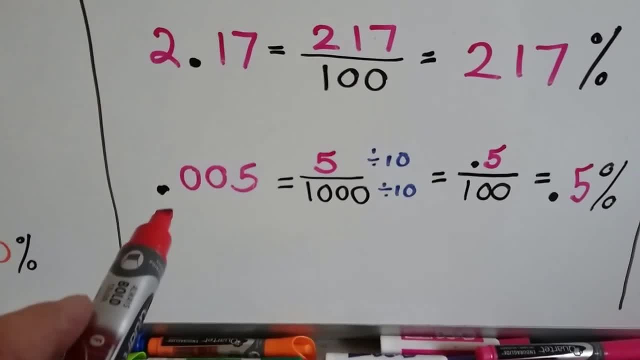 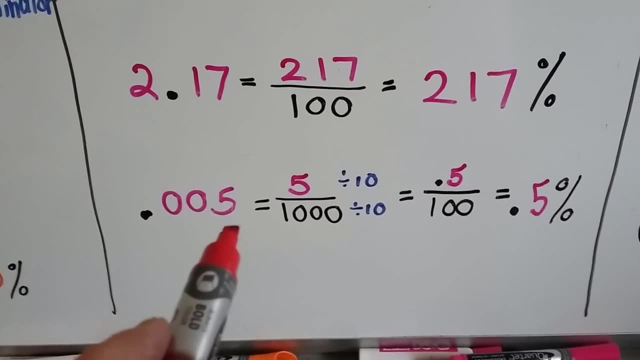 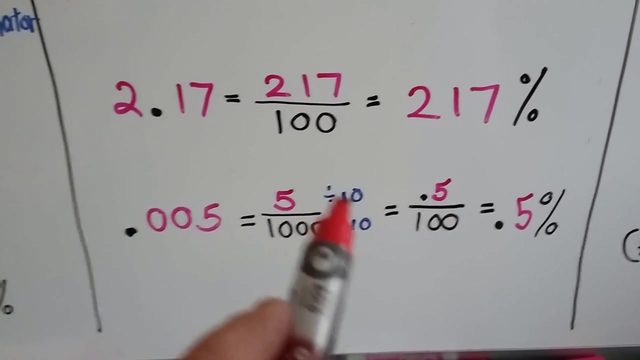 And here we have 5 thousandths. Now we saw this in the last video. How do you turn 5 thousandths into a percentage? Well, it's 5 thousandths. We have to divide the numerator and the denominator by 100, I mean by: 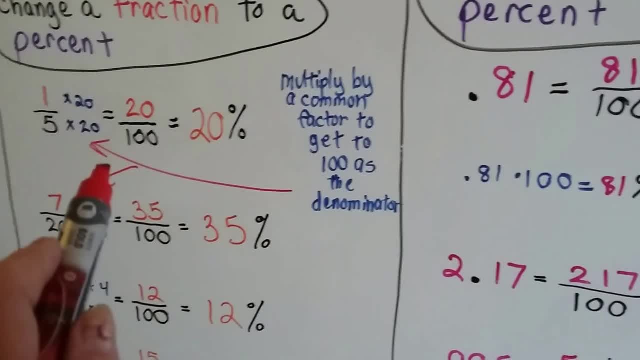 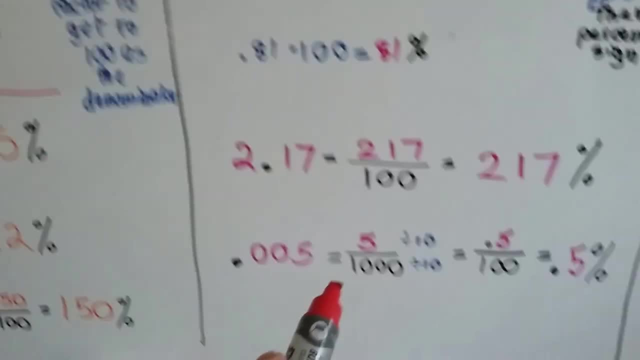 10, to get it to 100. Just like over here where we needed to multiply the 5 to get it to be 100 so that it could be the right fraction size to become a percentage, Over here we need to make it. 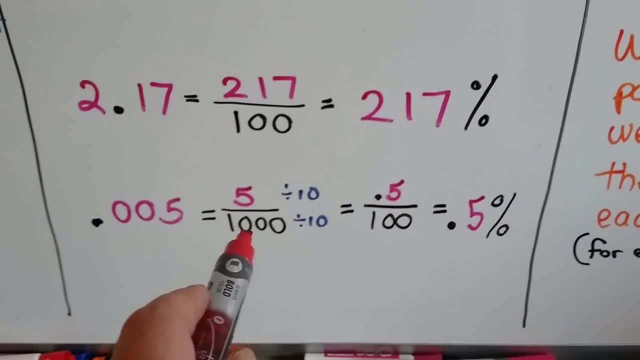 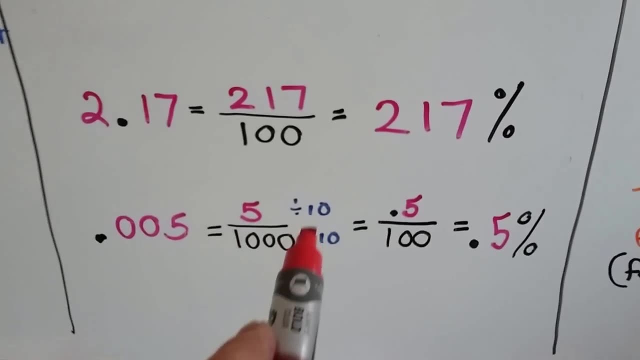 smaller, We need to get it to 100. And to get 1000 to 100, we have to divide it by 10.. Well, the numerator has to be divided by 10. But it's only a 5. So what happens? Well, when you divide, 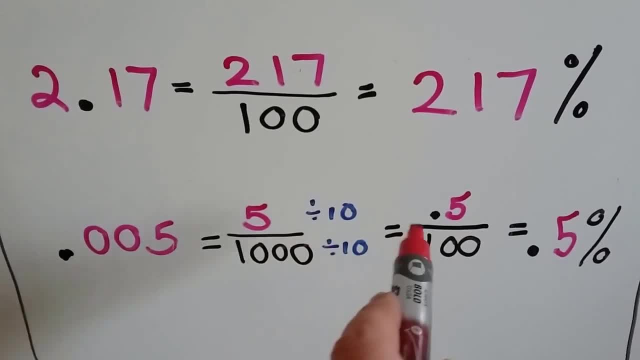 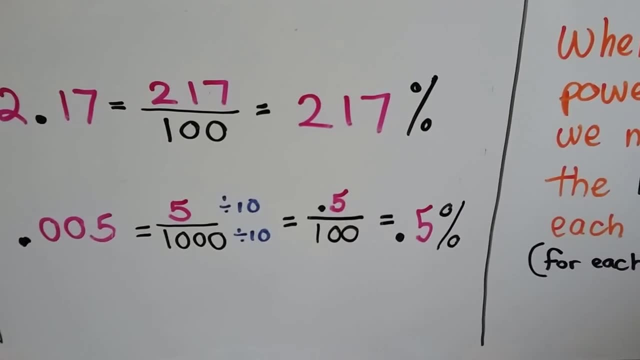 a 5 by 10, what happens is you end up putting a decimal point in front of it. So now we've got 0.5 over 100, which is 0.5%. See, So you can have a decimal and a percentage. 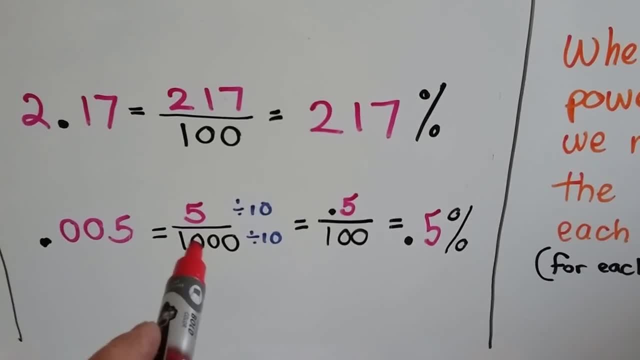 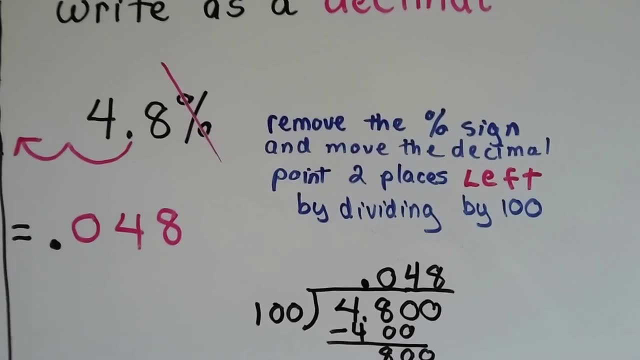 at the same time. But if you do, that means you're going into the thousands and ten thousands and stuff. Okay, If you wanted to write a percentage as a decimal, you remove the percentage sign and move the decimal point two places left by dividing by 100. 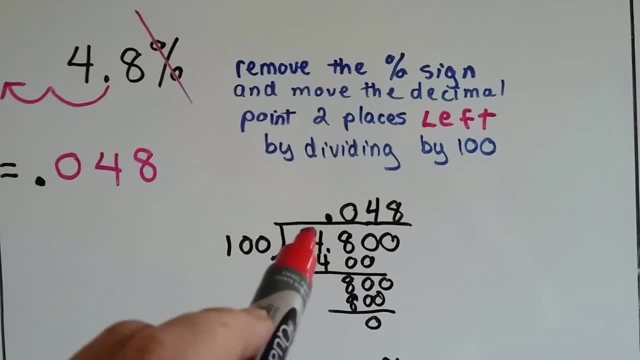 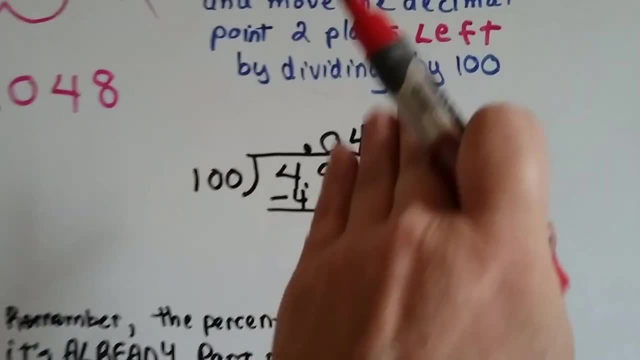 If we had 4.8%, I would do 4.8 and I would have the 100 as the divisor and I would do my long division. Can 100 go into 4? No. Can it go into 48? No, So I put a 0 up there. 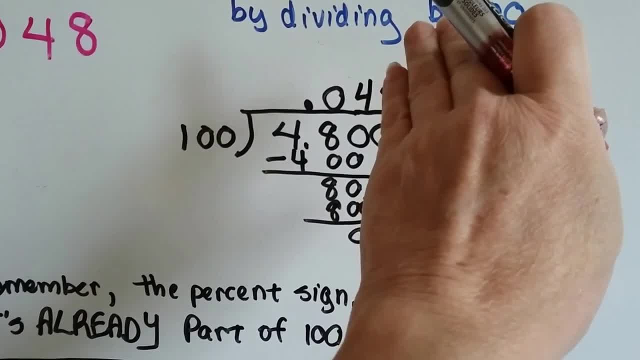 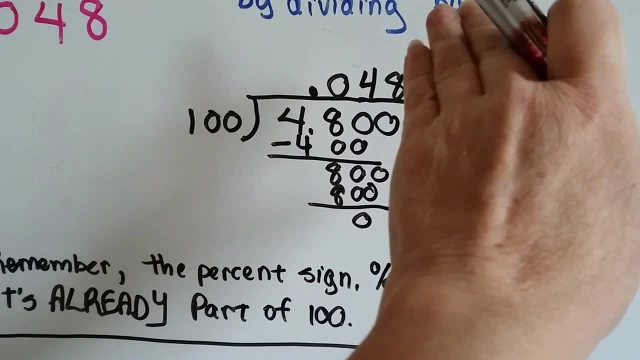 Can it go into 480?? Yes, four times. So I put my 4 up there. 100 times 4 is 400.. I did my subtraction and got 80.. Added another 0. And I said: how many times can 100 go into 800?? 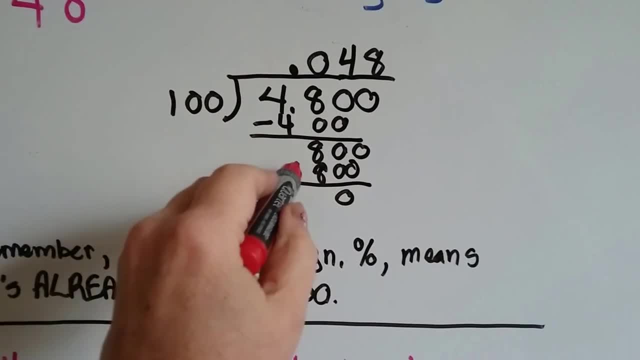 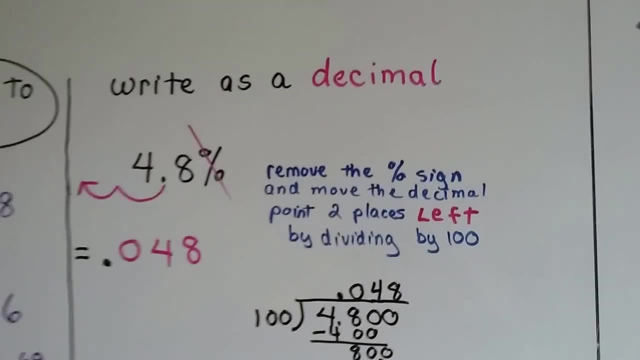 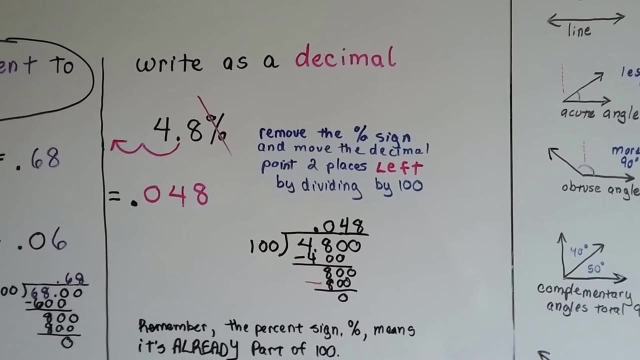 Eight times I did my multiplication and my subtraction and got 0.. And my answer is .048.. And that's what it is as a decimal See. So I turn 4.8% into a decimal by dividing it by 100.. 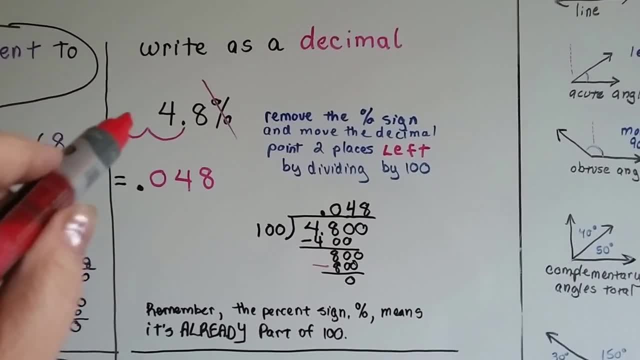 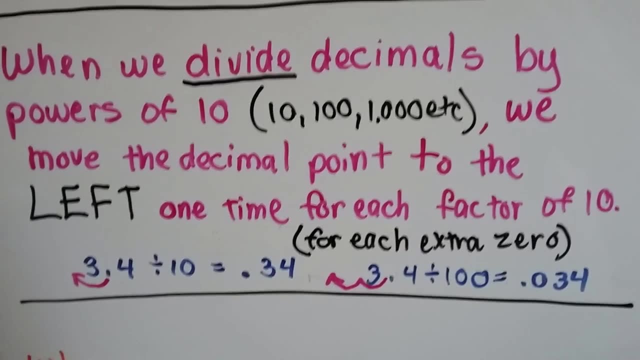 See, And that moved the decimal point. that way I had to add a 0 to hold the place. So when we divide decimals by powers of 10, which are, you know, 10,, 100,, 1000, those are the powers of 10.. 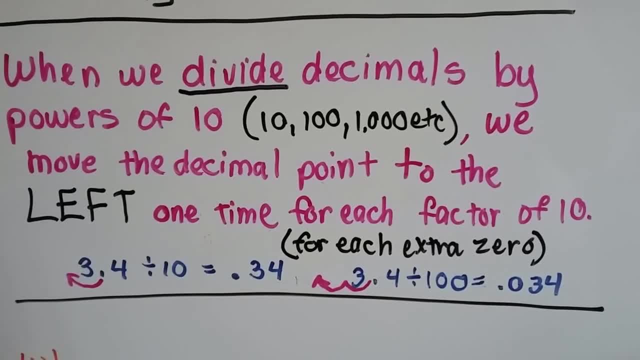 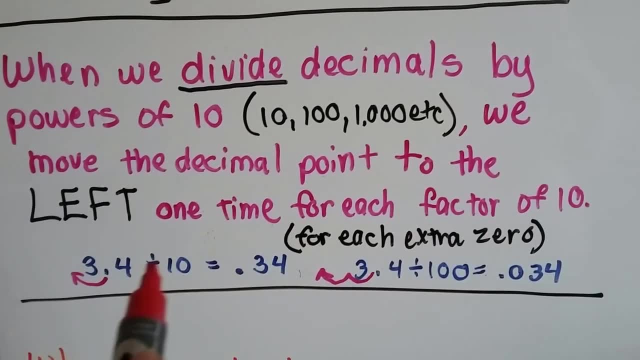 We move the decimal point to the left. Divide equals left. We move it left one time for each factor of 10, for each extra 0. So if you have a 10 that you're dividing by, you move it one time If it's 100,. 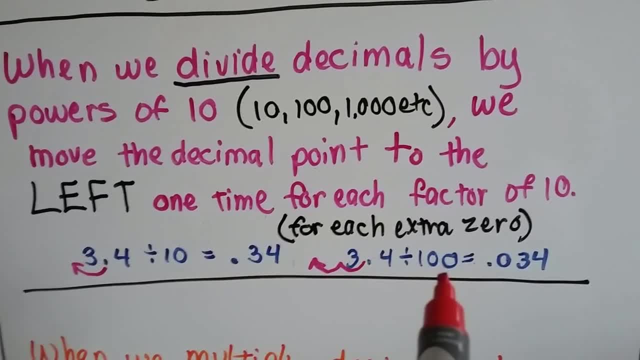 it's an extra 0.. You move it two times. If this was 1000, you'd have three 0s. you'd move it three times See. So, for each extra 0, you move it one more time. 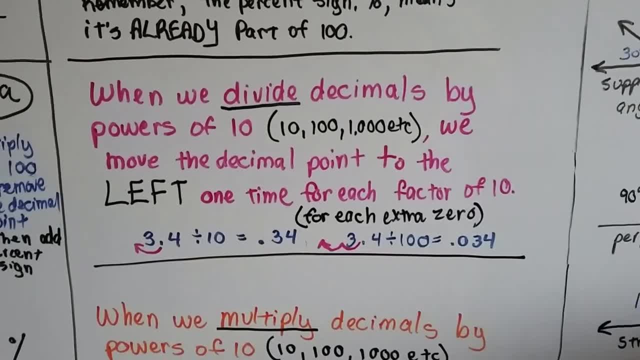 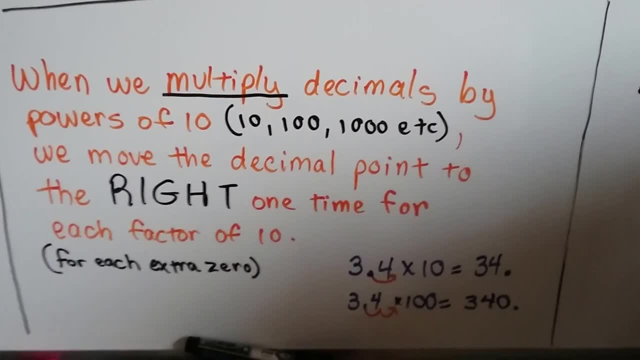 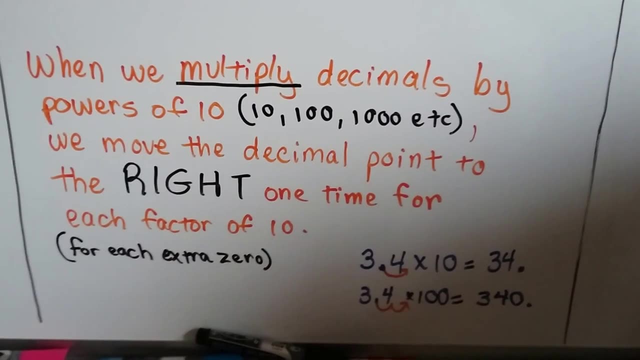 10 is one time, 100 is two times, And every 0 you add to that, you just move the decimal place again. When we multiply by decimals, when we multiply decimals by powers of 10, the 10,, 100,. 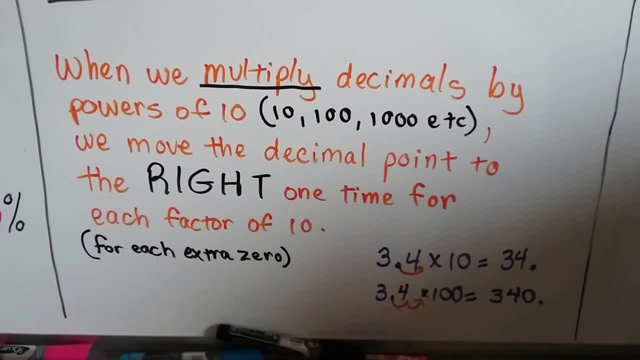 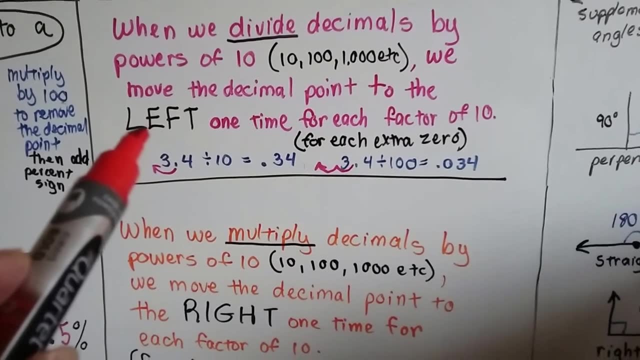 1000, etc. we're moving the decimal point to the right one time, for each factor of 10, for each extra 0.. So, dividing decimals, you move it left. Multiplying decimals, you move it right. OK.